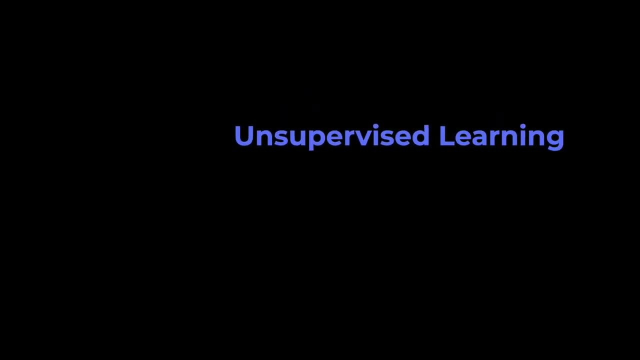 further ado, let's get started. In the last video, we learned about supervised learning, where the machine learning model learns by making use of labeled data. Now in unsupervised learning, we have unlabeled data Meaning. we have data, but we don't know the corresponding class or 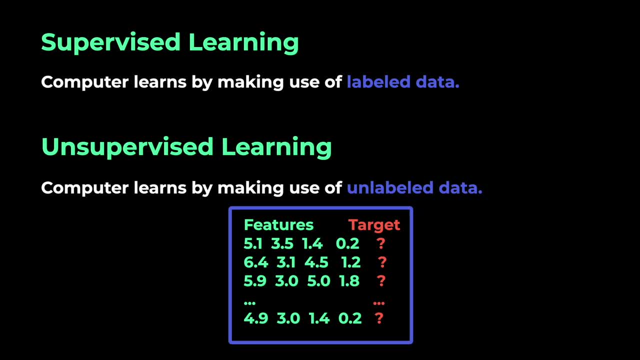 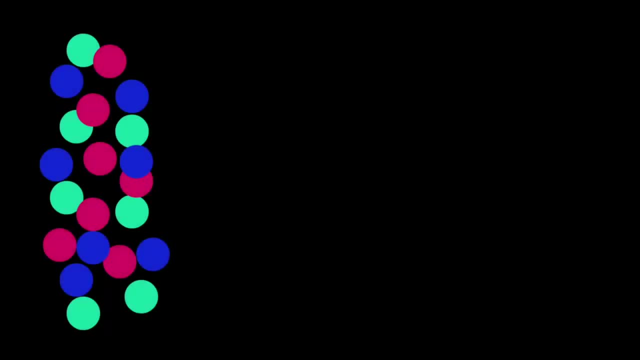 target for the features. This process is oftentimes more complex, but it has the huge advantage that it does not require upfront human intervention to label the data. But if the data isn't labeled, then how is the model learning? Essentially, the model is trying to figure out some kind of 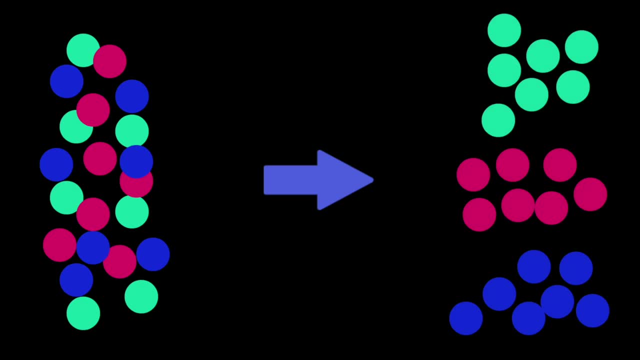 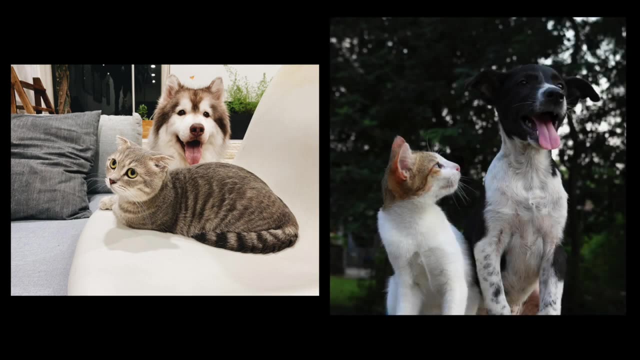 structure in the data and will extract the useful information from it. A popular example is object recognition, a common task in computer vision. Here the model finds similar looking objects and marks them without knowing its specific label. Each group has its own characteristics that 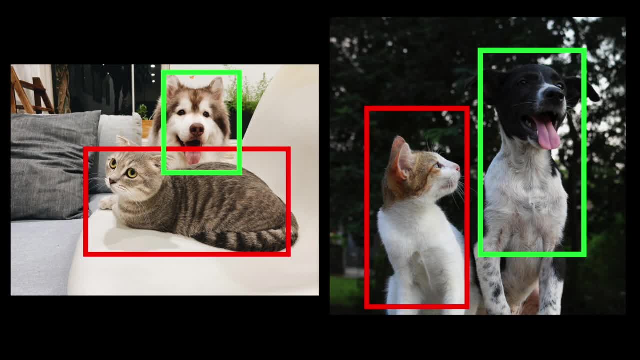 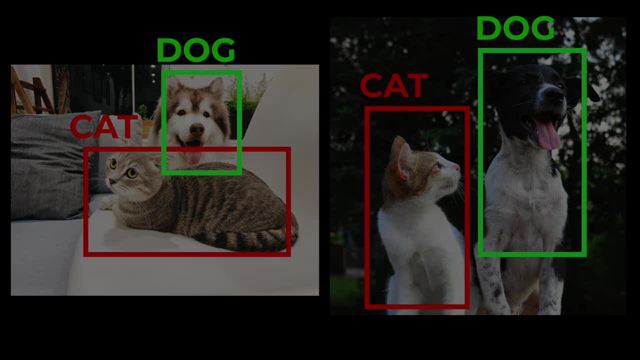 the model learns to identify and afterwards we can very easily define the associated label for this group. Now let's look at different applications of unsupervised learning. One of the most used applications of unsupervised learning is clustering, which is the process of grouping. 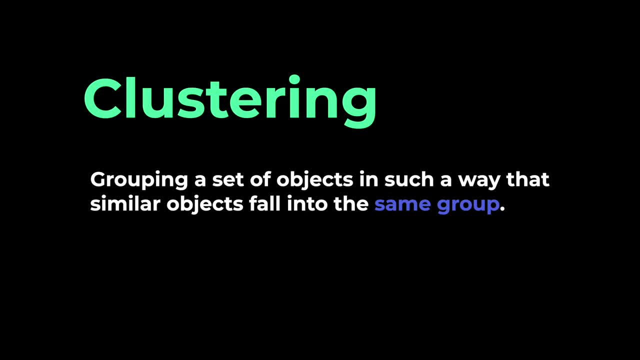 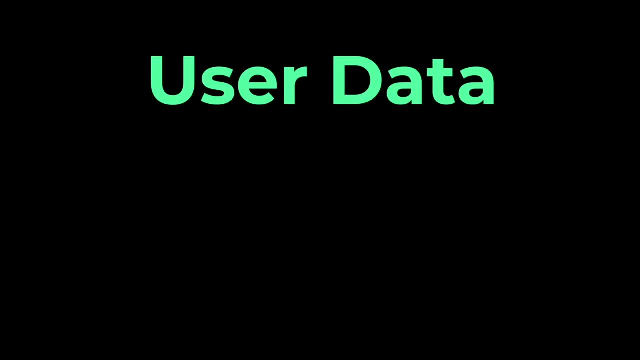 and set of objects in such a way that similar objects fall into the same group. Imagine you are the founder of an e-commerce website. For each user you could somehow collect the age and income, but other than that, the user stays anonymous. Now you want to determine if the user is likely to buy. 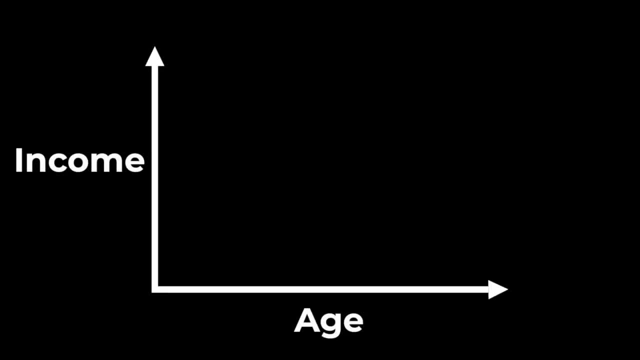 your product or not. This can be done by analyzing the data and identifying two possible clusters: One cluster for the group that is interested to buy and another cluster for the group that is not interested. Of course, this example is a little bit oversimplified and real world data oftentimes 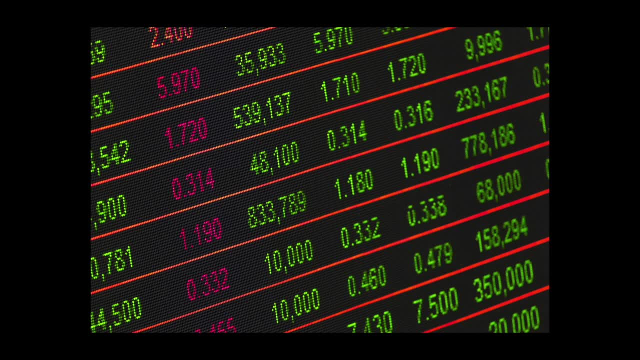 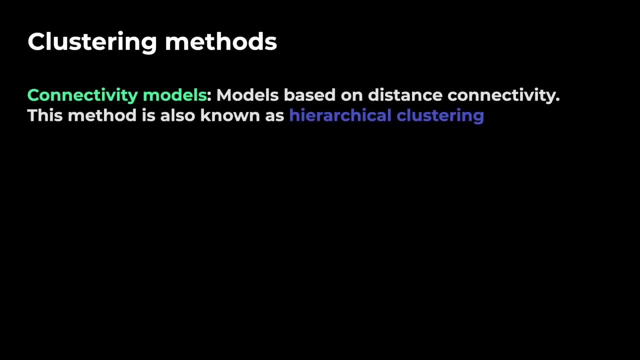 does not look that simple. That's why the model needs to use a more sophisticated way to find the clusters. There are different approaches, For example, connectivity models. Here we build models based on distance connectivity. This method is also known as hierarchical clustering. 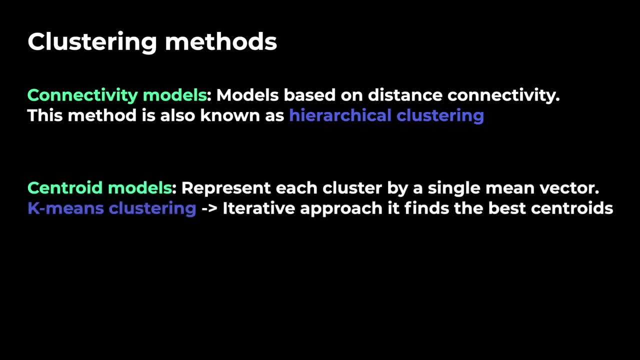 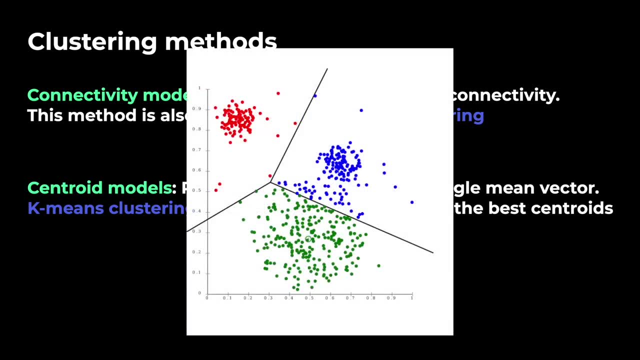 Centroid models represent each cluster by a single mean vector. A common example is the k-means clustering algorithm that represents each cluster with its mean vector, also called centroid. In an iterative approach, it finds the best centroids and assigns all the surrounding data points to. 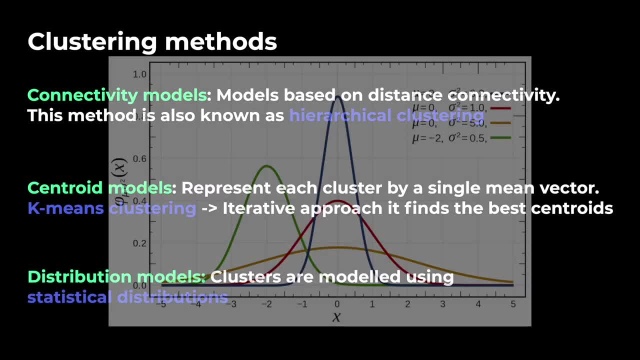 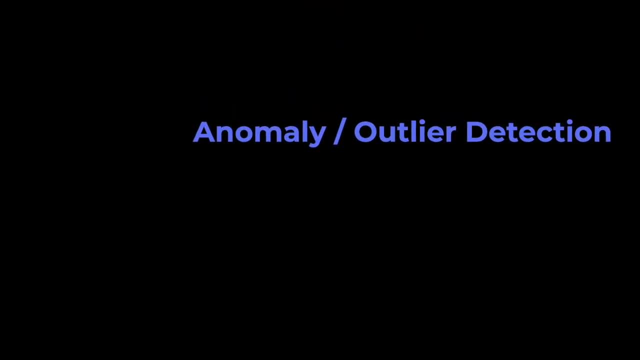 this cluster And we have distribution models Here. clusters are modeled using statistical distributions. Another possible application is outlier detection. Oftentimes, datasets contain a few samples that fall out of the typical range. These samples are called outliers. If we were to train a supervised model with this dataset, the outliers might confuse the model and 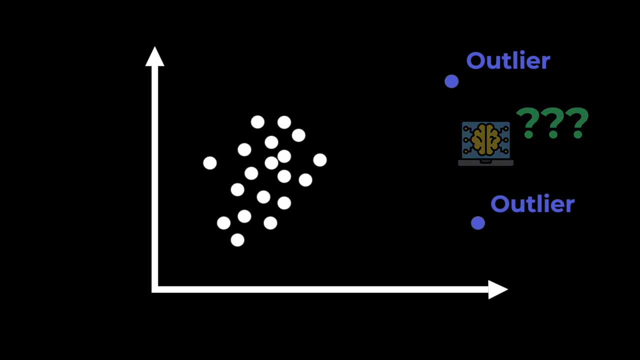 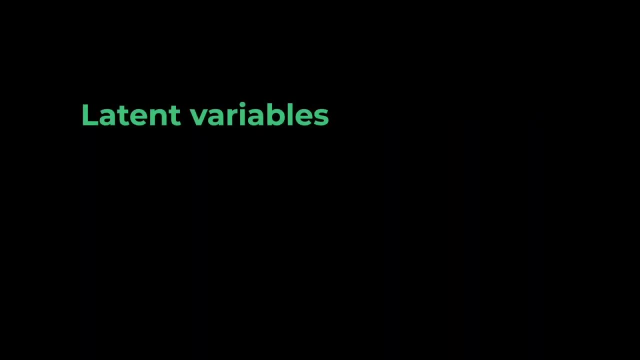 lead to incorrect results. That's why oftentimes it makes sense to identify and remove these outliers with an unsupervised learning technique before moving on to a supervised learning task. Another application is latent variable modeling. In statistics, latent variables are variables that are not directly observed, but are rather inferred from other variables. 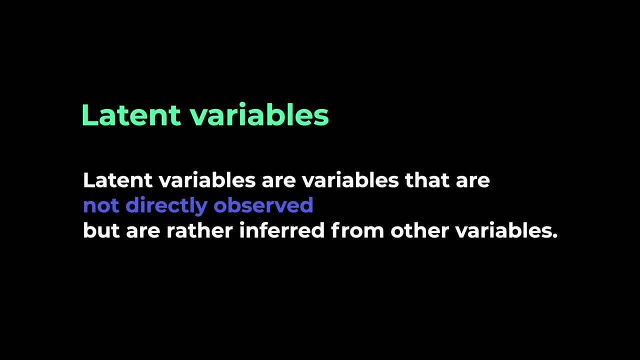 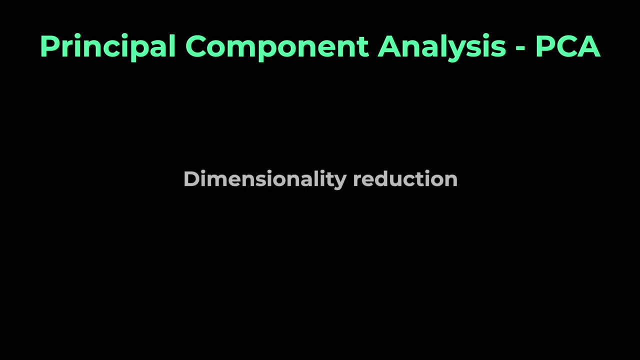 In this example we can see that latent variables are variables that are directly measured. Mathematical models that aim to explain observed variables in terms of latent variables are called latent variable models. A popular method in this category is principal component analysis, or short PCA. PCA is commonly used for dimensionality reduction. It computes the so-called 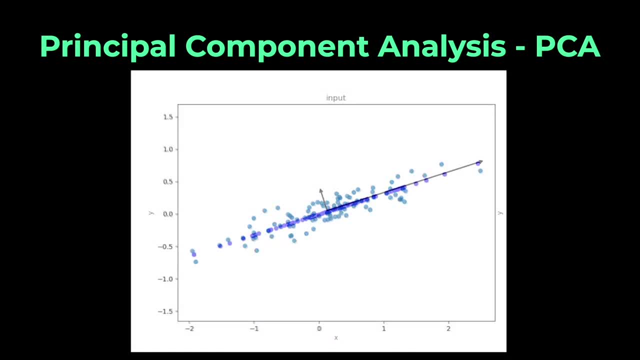 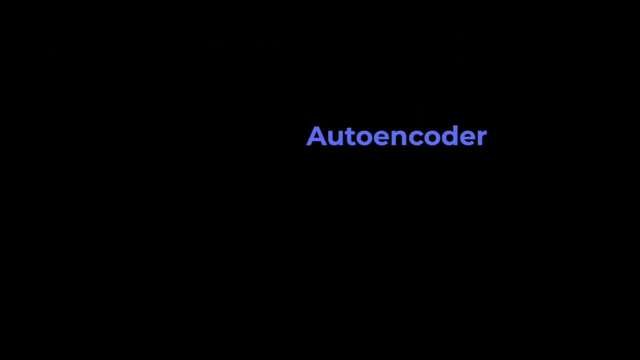 principal components and then transforms the data by projecting all data points onto these new axes. In this simple example, we end up from a 2D space in a one-dimensional space on the line, but of course this can be used for any number of dimensions. Neural networks can also be used for 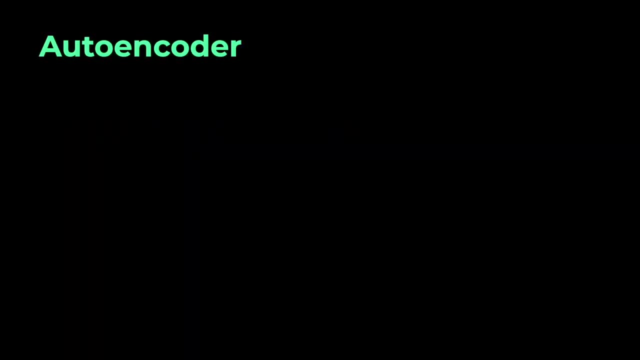 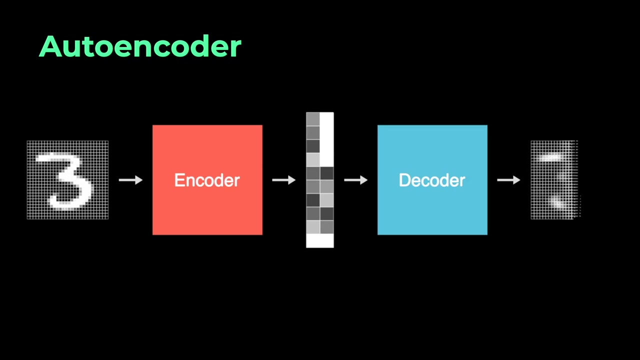 many different unsupervised learning tasks. One particular neural network type is the autoencoder. Autoencoders have an encoder part that encodes the image to get a low-dimensional embedding of the image, and after that it gets decoded again by the decoder with the goal to reconstruct the 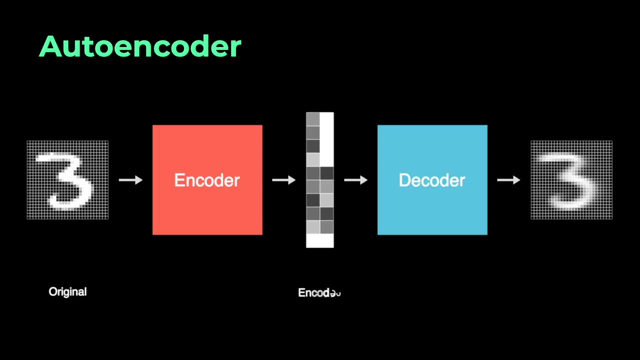 original image as good as possible. During this process, there is no need to know the actual label of the image. But what can this be used for? Two possible use cases are: denoising the image By encoding the image and learning meaningful features of the image to reconstruct it. 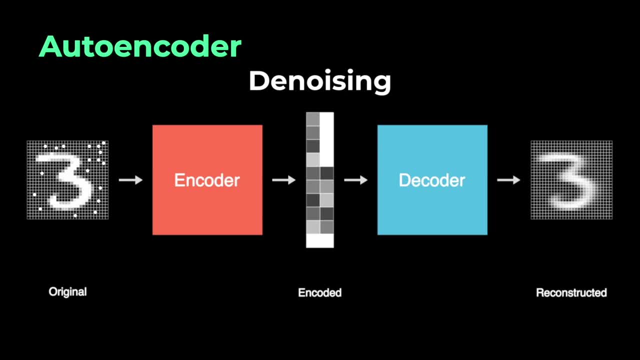 we can remove noise or other unwanted things from the image, Or we can do image and video compression, where only the encoded representation is used to be sent over a network from one end and on the other end it gets decoded again to see the normal image.